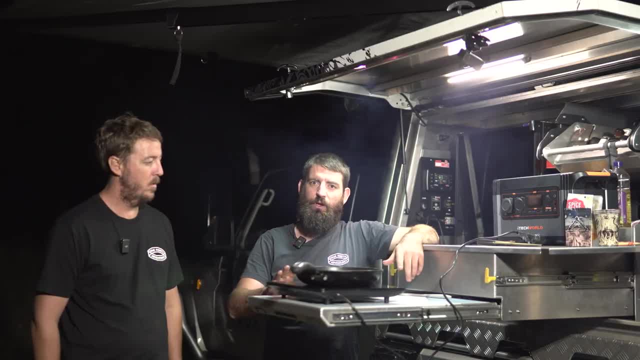 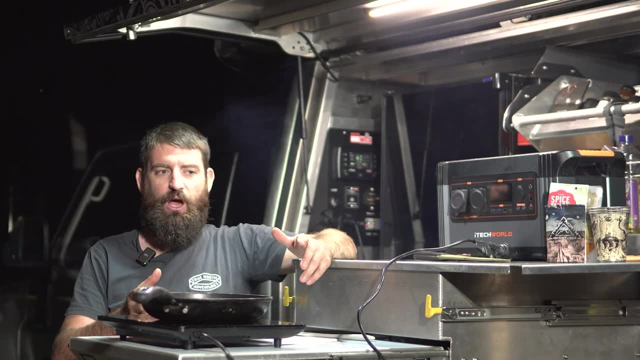 Hey guys, tonight we're going to show you how we cook on the induction cooktop. We get a lot of questions about it, What battery setup you need, how big your batteries need to be, how big your inverter needs to be. So we're going to put that to rest. We usually cook on the car, but tonight 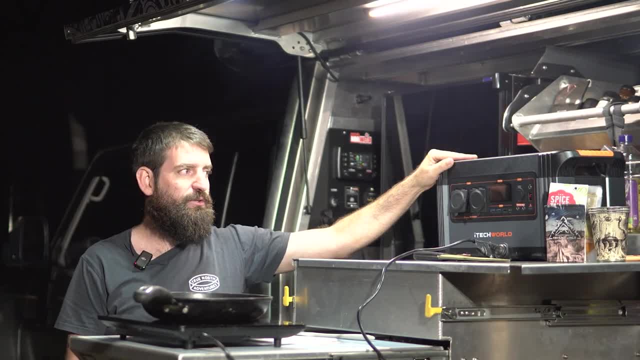 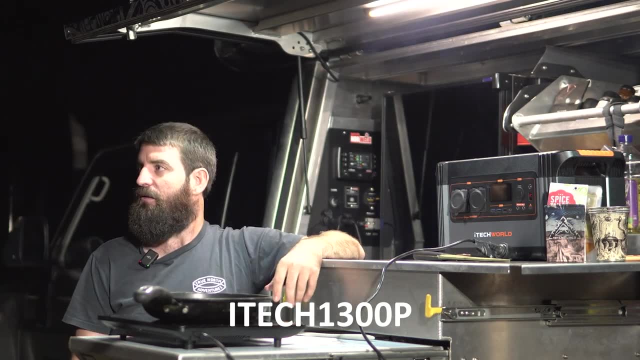 we're going to use the 100 amp hour battery here. It's a portable battery. Anyone can buy it and just throw it straight in the back of their car and you don't have to have a massive big setup in your car and you can move it around. You do need to ensure that it's got the capable inverter. 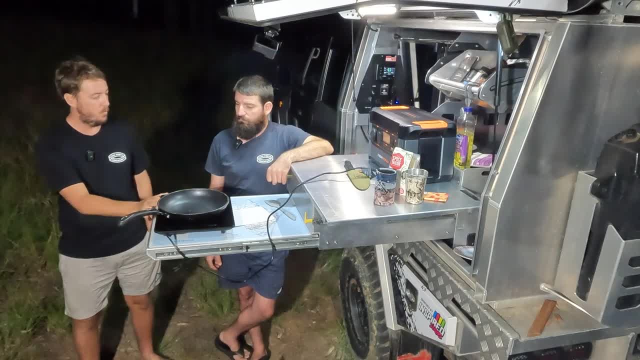 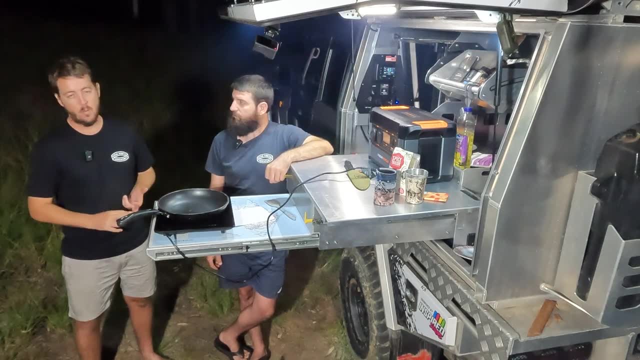 Now this cooktop- they're not expensive- this induction portable one and they'll cook up to like 2,000 watts, but you don't need that. You need to cook it about 8 to 900.. So you're going to want an inverter, like a continuous pure sine wave inverter, of at least a thousand. 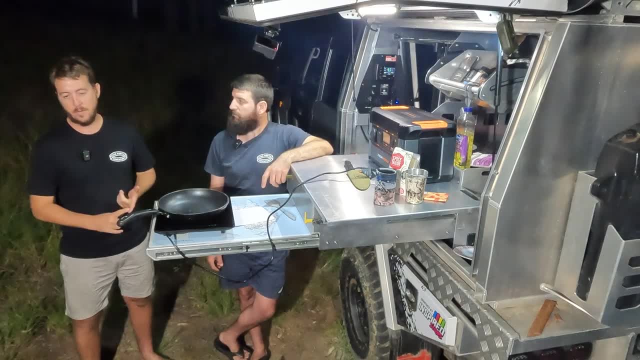 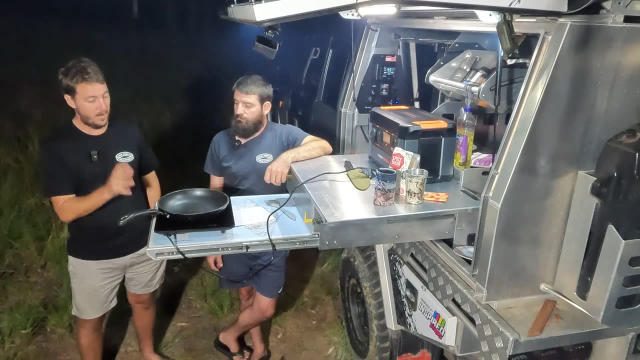 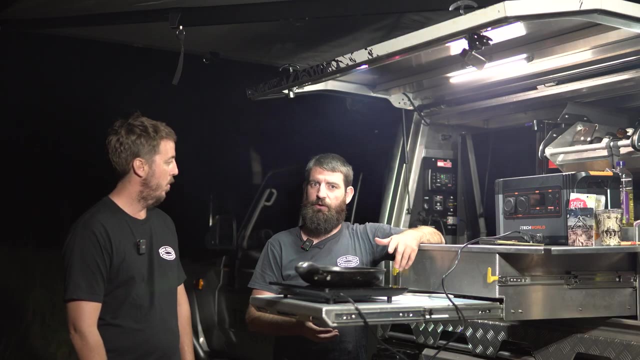 This iTech World one. it peaks at 2,000 and has a continuous output of 1,300.. It's going to suit what we're doing, Really great display so we can monitor a standard meal that we cook for camping. what sort of drawer it's going to have? We get a lot of questions: how much power? 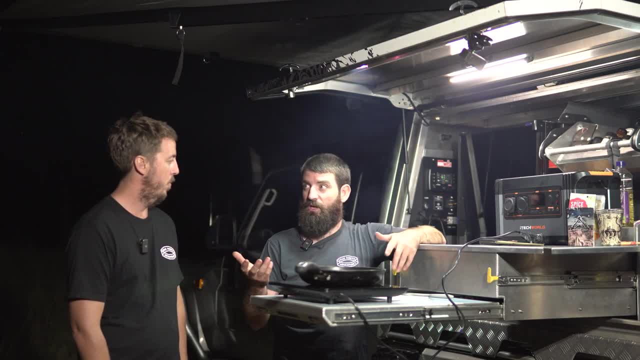 do you use cooking a meal? Yeah, So it's a really standard meal. we cook probably a standard meal. we think a lot of people cook camping. We'll be able to tell you from start to finish, from 100%, how much power we draw. Yep, let's do it. Let's go Get a beer, mate. I'll get two, you want one? 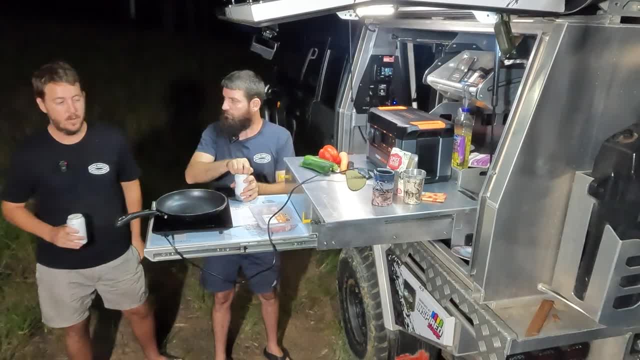 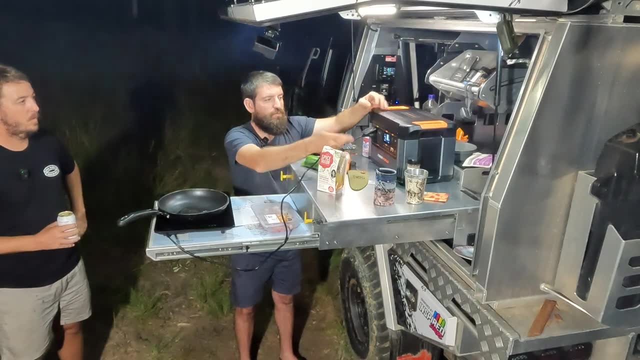 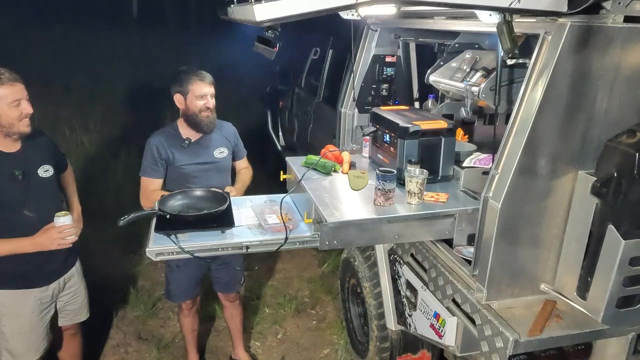 Yeah, please. The meal we're cooking tonight is just a camp curry Power on Sweet. We're at 100% on the screen there. If you can't see it too bad, You're just going to have to believe us. So we're going to go down to about 1,000 watts. I'm actually going to turn that down. 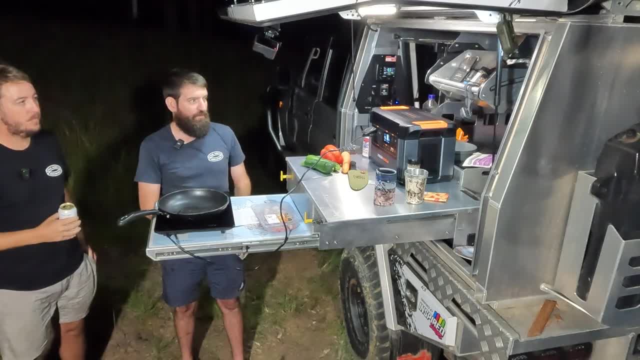 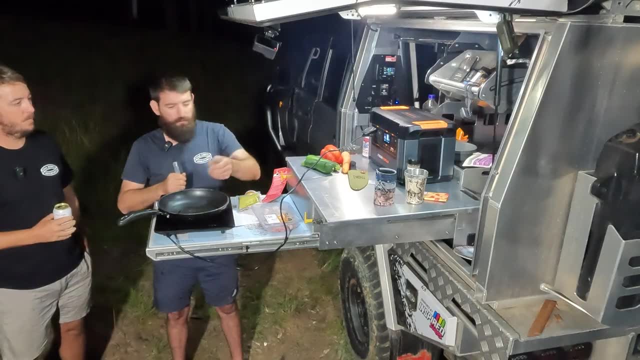 to about 800 watts on the inverter. there We're drawing about 1,000 watts out of the battery. So there you go. You can see it kicking in and out. as the induction kicks in and out. Cool, So we're. 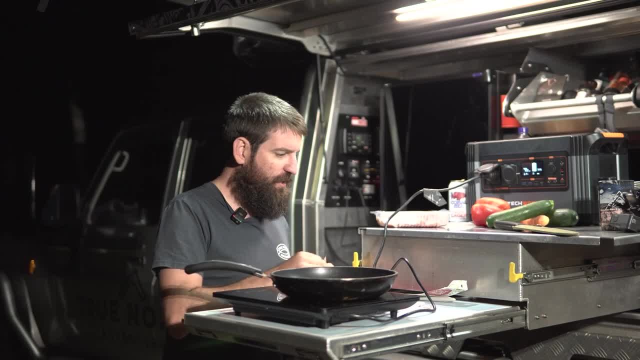 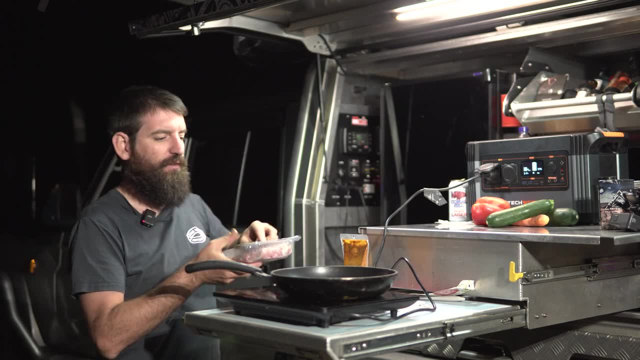 just throwing some spices in there, Cook them for a couple of minutes now. Then we're going to add some chicken, Cook lightly for a couple of minutes and then put the base sauce in after that, Still at 800 watts on the induction cooktop here. I don't think I'll change that throughout the cook. We've used it a. 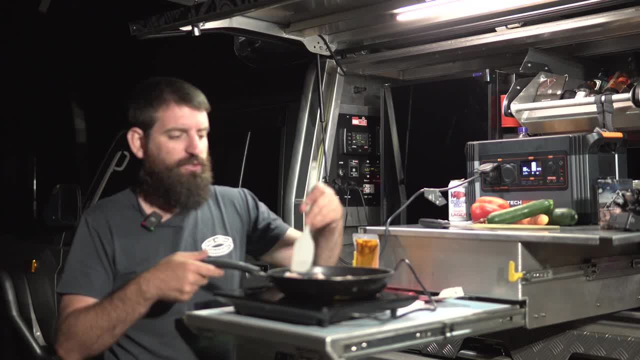 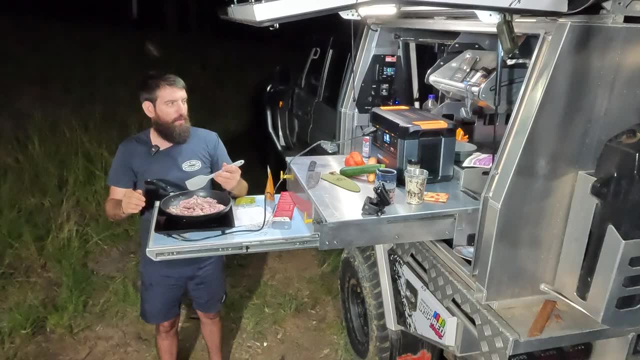 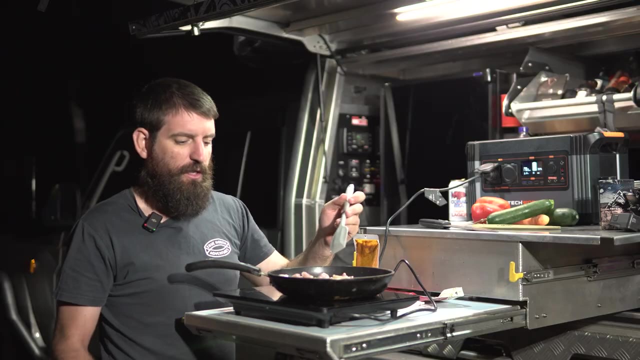 fair bit and find that 800 watts is a pretty good cooking temperature. On the inverter we're drawing about, it pulses in and out, So when it kicks in we draw about 1,000 watts and then it will drop out for about half that time again and draw nearly zero watts. So this induction cooktop 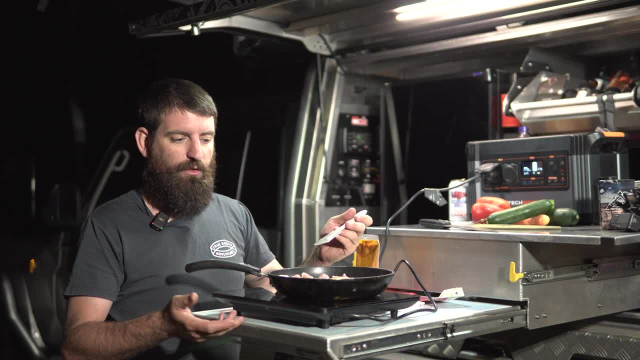 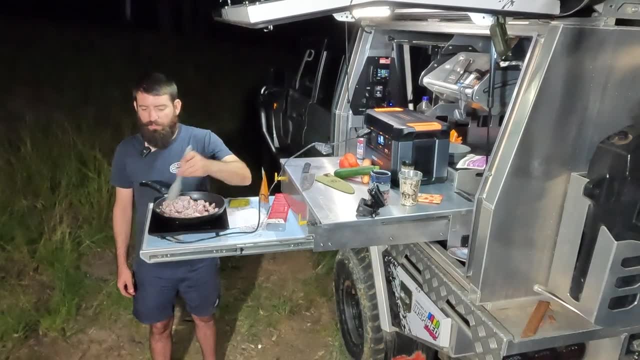 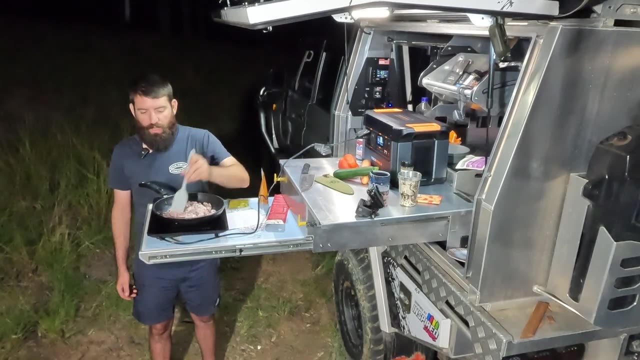 here is just: yeah, It's a Breville induction cooktop. I mean, you walk into Good Guys or something like that and you're going to have five different options. They're all around that $100 mark. They all do the same job. We've used this Breville one for well and truly over a year now- nearly two years. 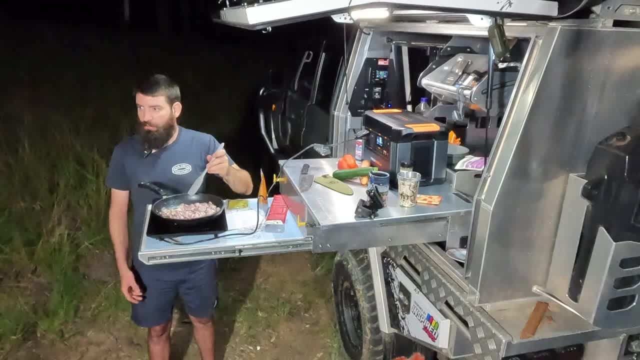 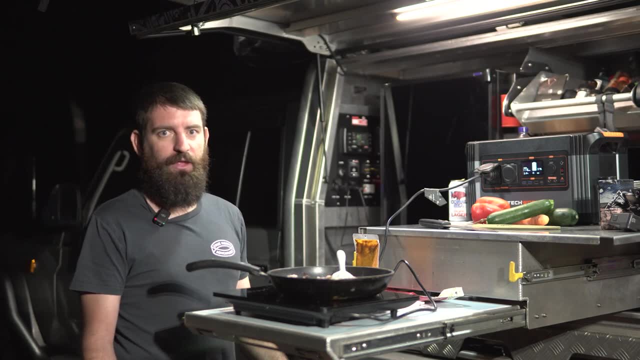 And it's been in the back of the car bashing around, going up and down dirt roads and it's still going. So, yeah, if I had to recommend one, this would be it at the moment, But I'm sure any of the other. 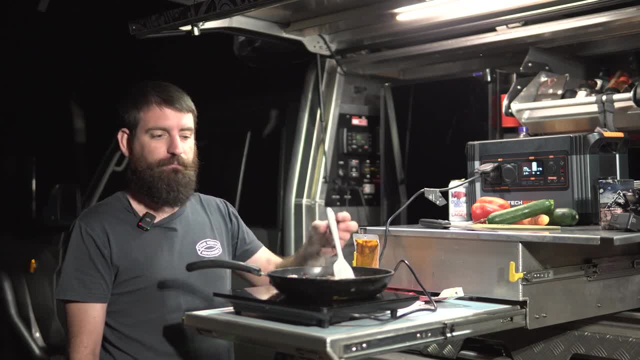 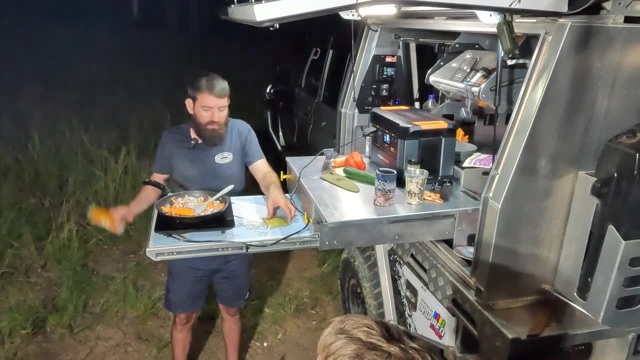 $100-ish sort of induction cooktops are going to do the same job. So we've just browned that chicken off and thrown in a couple of the carrots, because they'll take a bit longer to cook. Now we've got our base sauce to put in there, So I'm just chucking in a couple extra veggies now. that won't. 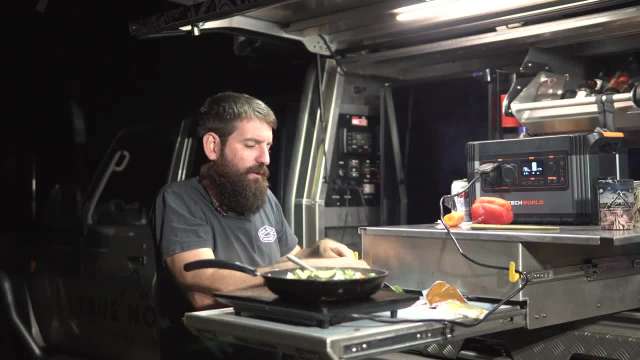 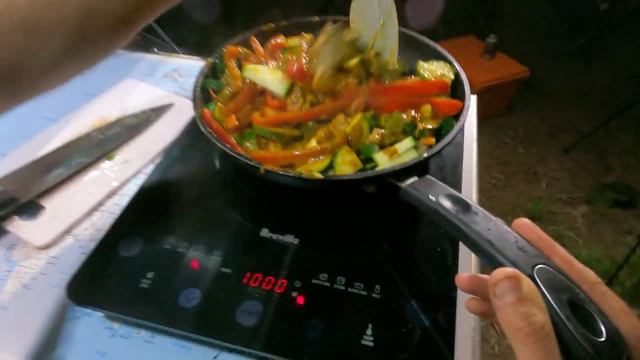 take as long to cook as the chicken, And then we'll throw the main sauce in and we're nearly done. Man, it smells good, eh, Oh, sensational. It's actually juicing up as those veggies cook down a bit. So what do we reckon about the chili mate? This is really good, isn't it? 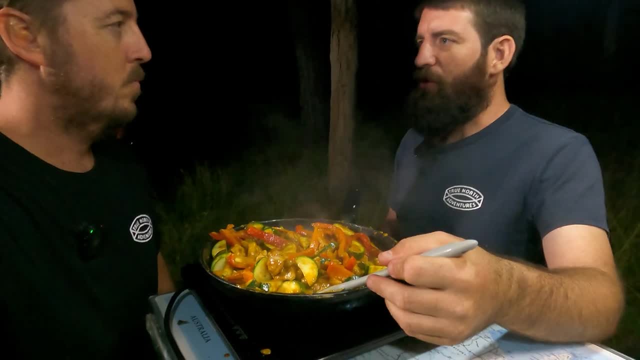 Is there chili to go, or Yeah, actually I reckon a curry should make your nose water. Yeah, just a little bit. Just a little bit. yeah, I mean, you don't want to not be able to taste the food. 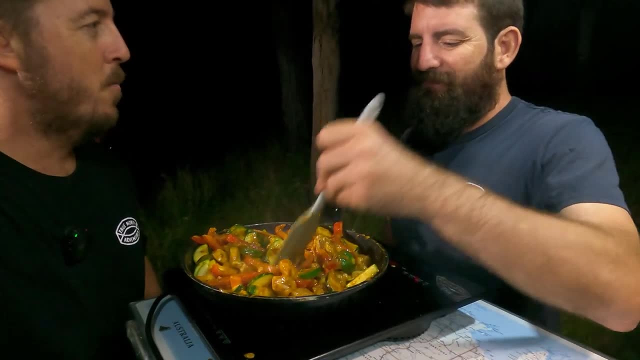 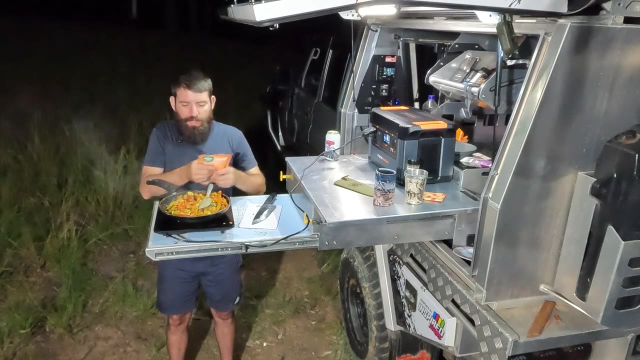 When you start questioning if you like it or if it's too hot, it's the right amount. Yeah, you just like the water? Yeah, I agree. Yeah, Yeah, Yeah, But the answer is I do like it, Right, so we're going to add a bit of rice to this curry. 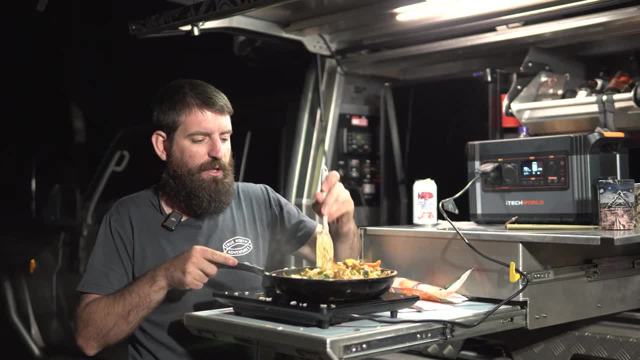 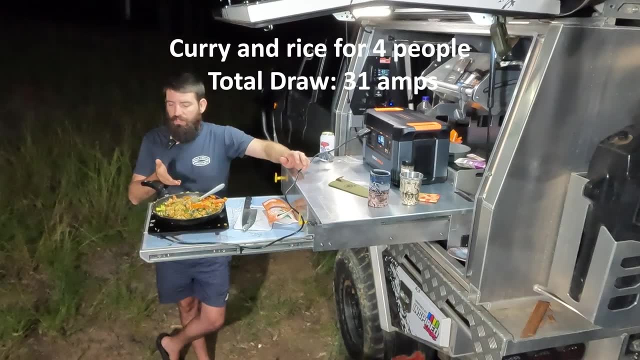 I'd say rice has had about 45 seconds a minute to heat up a bit. I'm going to turn that off, So that's amazing. We've got a meal done That'll easily feed four people. I mean, it's three of us tonight. 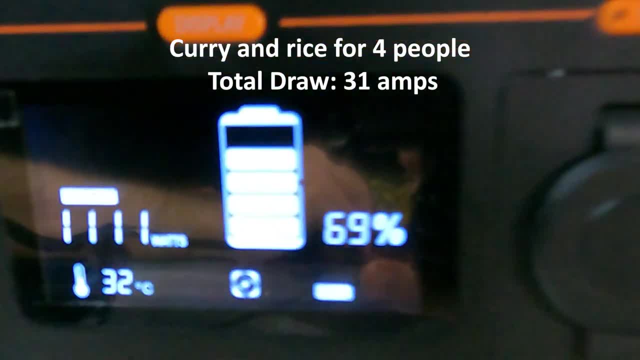 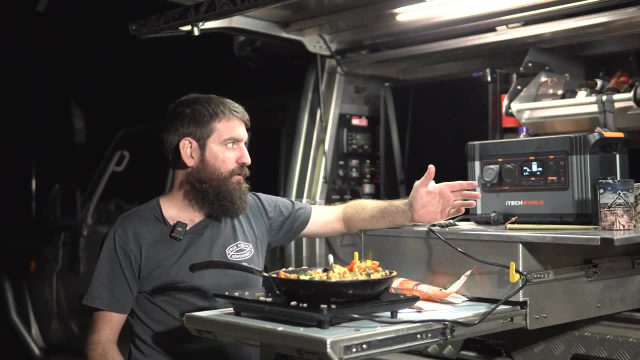 We've used just over 30%, So it's 68% on the battery. So if you were going to cook that three times a day, you were going to cook breakfast, lunch and dinner. you're obviously at 100 amps, So if you've got no way of charging your battery, 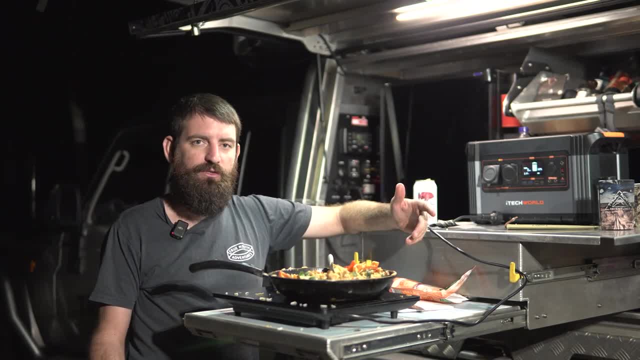 through the day. your battery's only going to last one day. If you've got solar set up or you're driving or something like that, you're going to be able to cook one or two meals on it in a day, no problems. Still run your fridge. still run your. 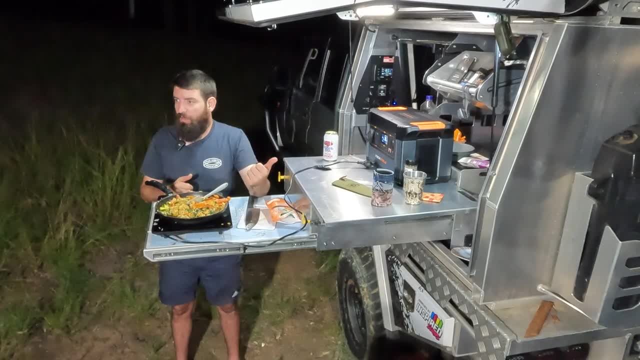 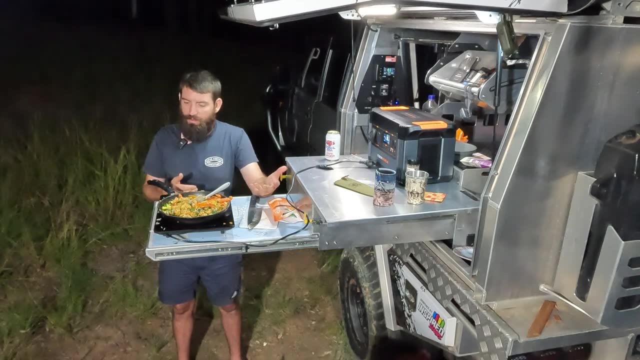 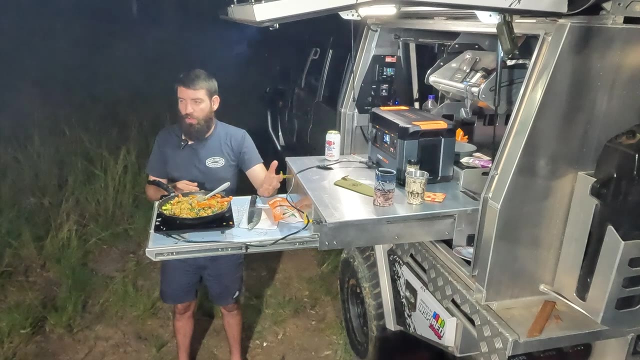 LED lights and have no problems at all. That's on a 100 amp hour battery. If you've got a bigger setup with a 200 amp hour battery, obviously more capacity. you could do it more times without charging it. But it's a pretty viable option And in a small form factor like that you can throw on. 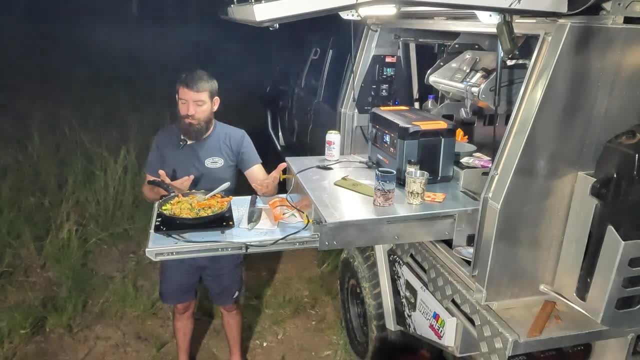 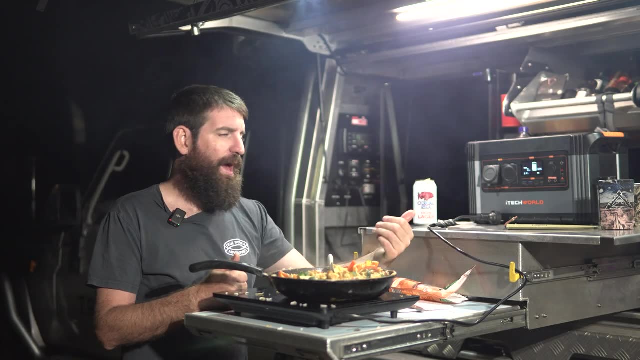 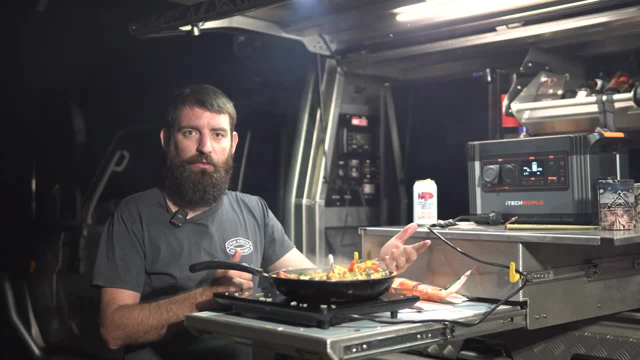 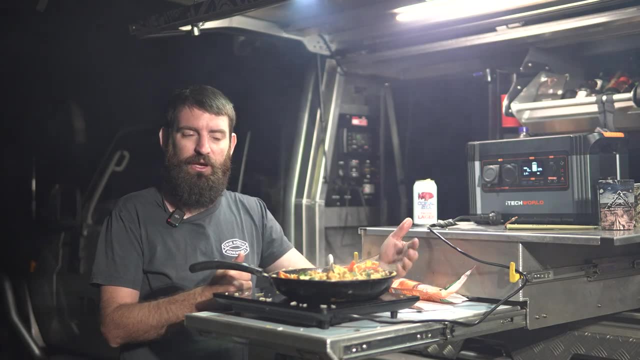 Constantly rechargeable, whereas something like a gas bottle- if you're away for a while, I suppose take a long time to empty it, But it is something that you have to constantly monitor and worry about. emptying A battery like this, you can constantly fill it up, just with solar. So 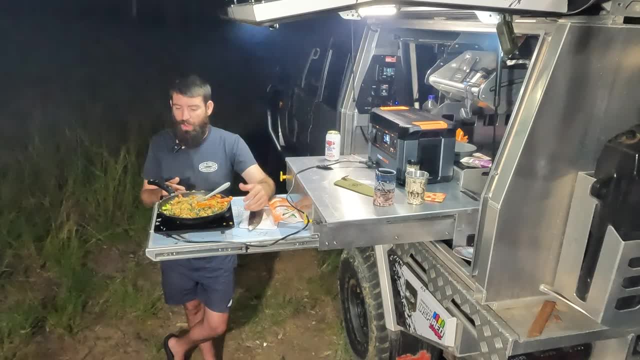 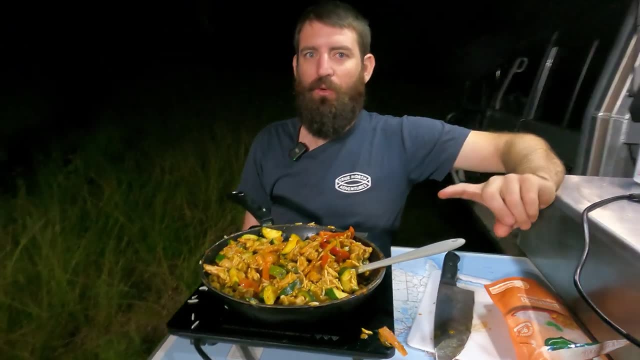 there's some great advantages to it, Probably our preferred way of cooking when we're in a hurry on instant heat, easy setup, We love it. So definitely don't judge me on my cooking. If you've got any questions, chuck them in the comments below. We'll answer them. 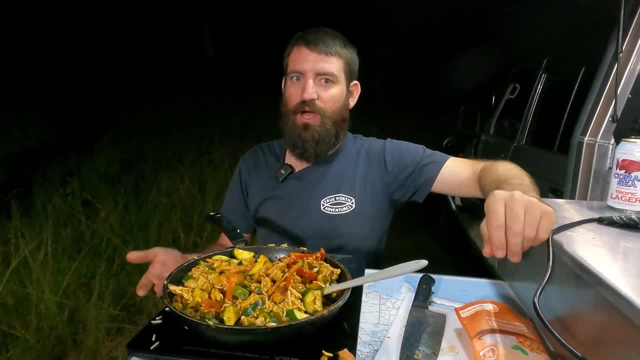 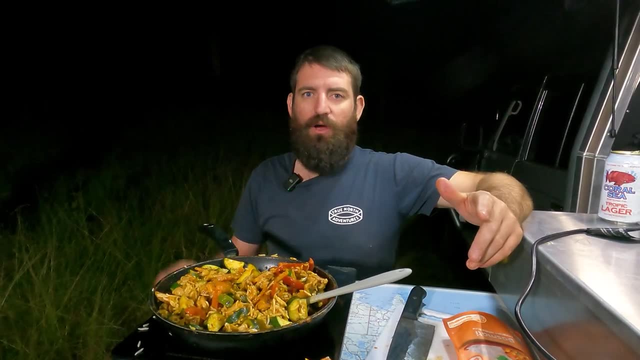 And if you want to support the channel, if you like this, if you want to see more of this, let us know. It's definitely different to our usual content, which is trips away, But if you want to support us, I mean watching is the best thing you can do, Like subscribe, all that caper. 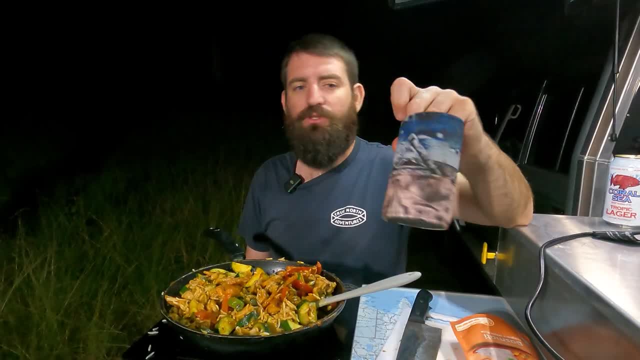 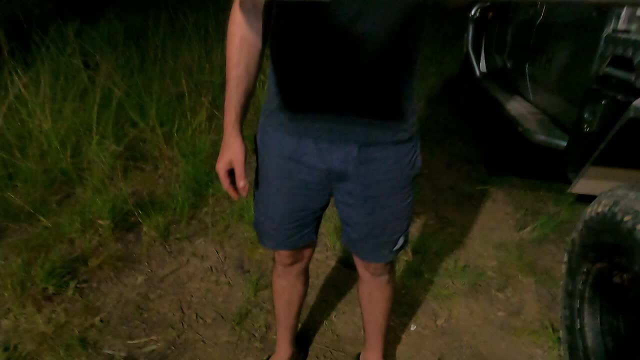 But if you really want to help us out and you want some cool stuff, we've got True North Adventure stubby coolers shirts, True North Adventure shorts- all on the website truenorthadventurescomau. Jump over there, Have a look around. Thanks for watching. 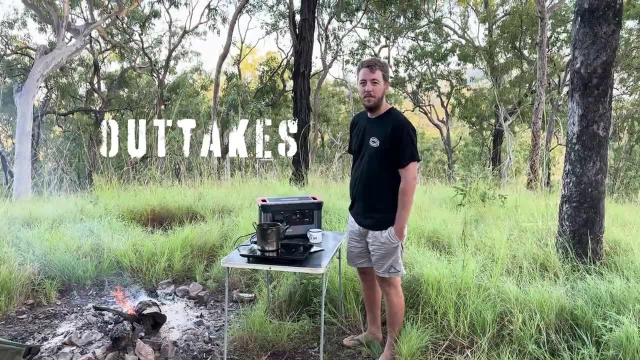 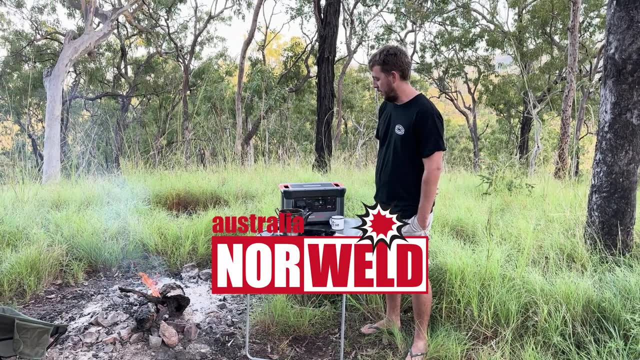 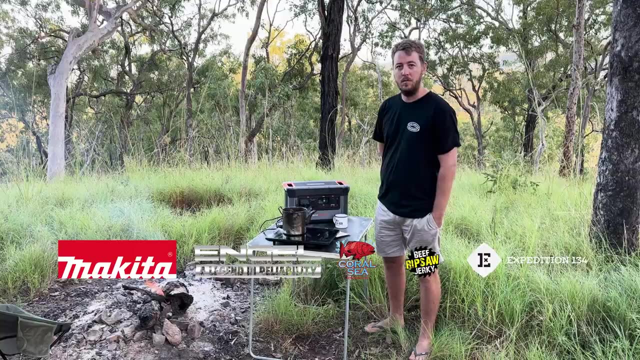 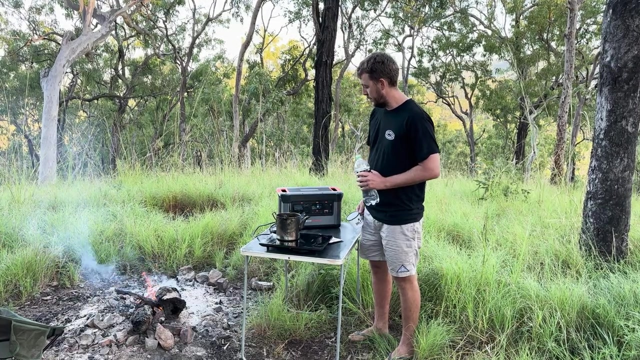 Go Morning, We're doing our coffee. Oh, we're doing our induction. I'll go again. Yeah, okay, Morning, It's coffee time. We're going to test the induction on cooking Measure. the Hang on The morning's not good eh.